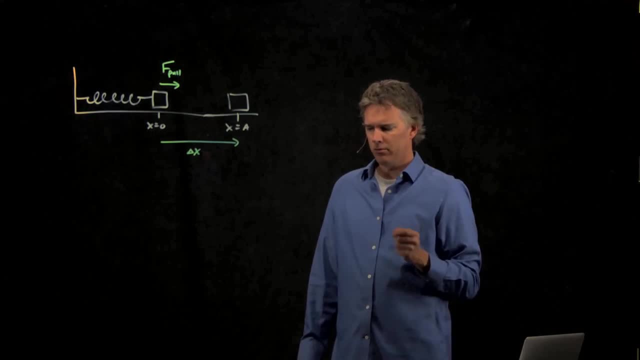 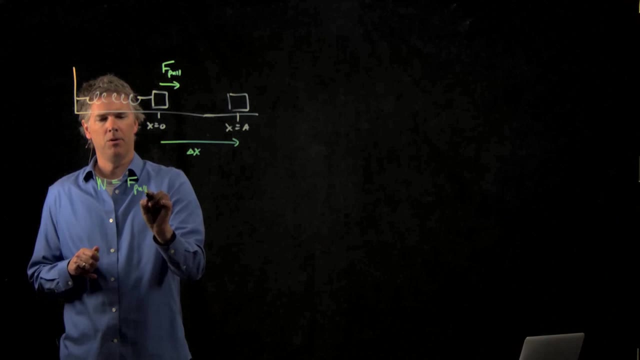 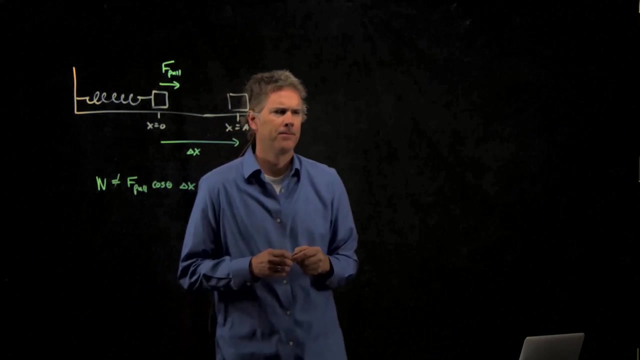 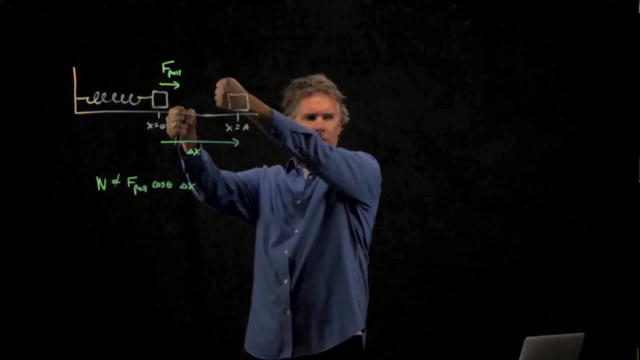 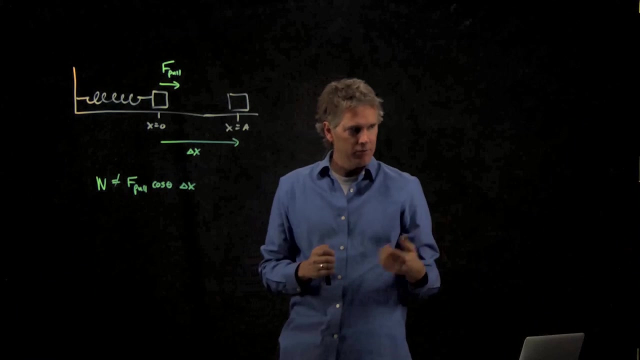 So we can't just write this. Work is not f pull cosine theta delta x. Why can't we do that? We can't do that because as you pull on the spring, it gets harder and harder to pull on the spring. Okay, the force varies as you go, And so we can't just write that. We have to in fact do the integral. 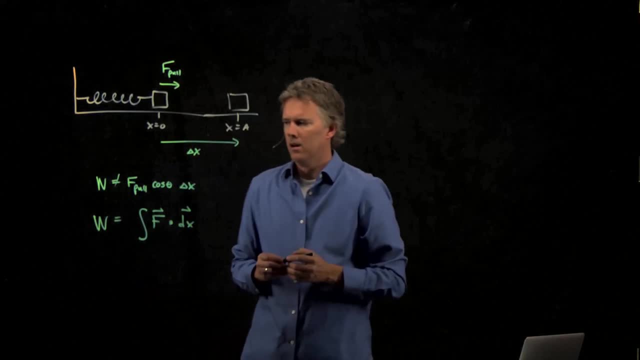 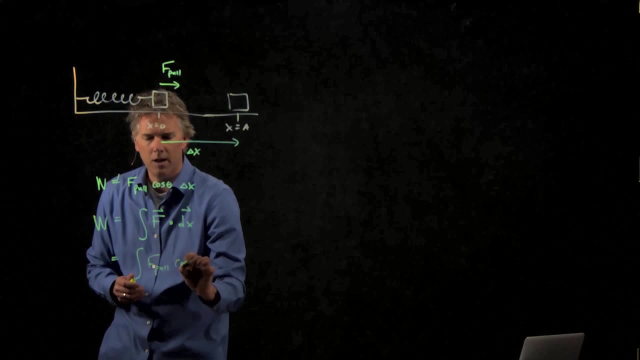 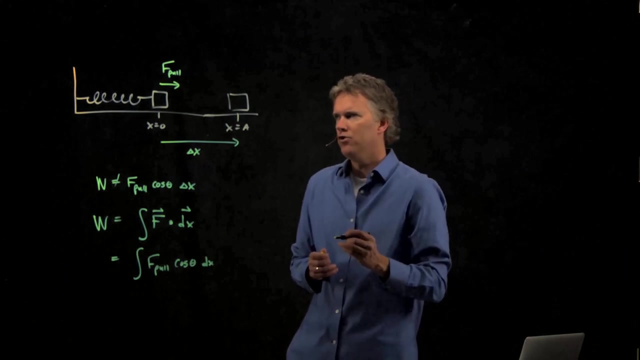 Okay where, this is our good old dot product right there. All right, Let's do the integral. So we've got integral of f pull, cosine theta dx. But we know that f pull just has to be as big as the spring force itself. kx. 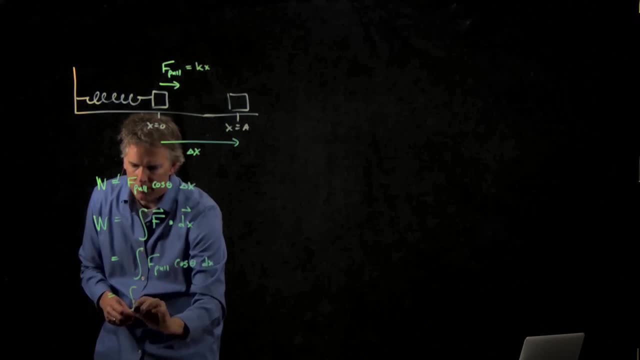 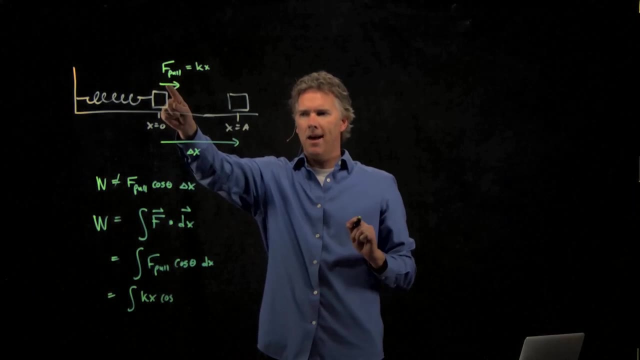 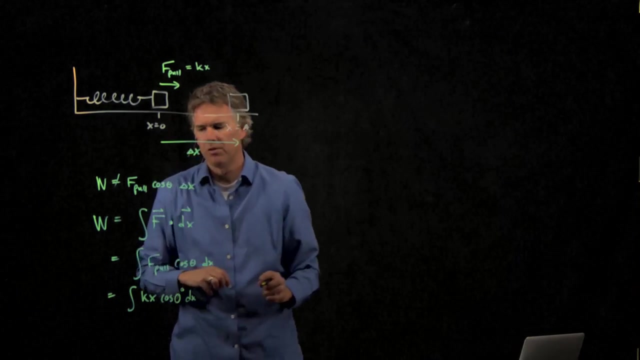 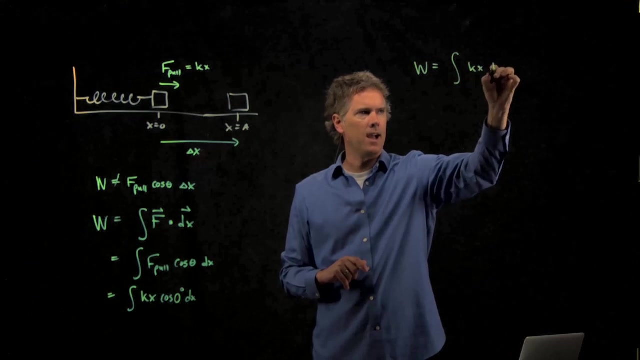 And so this whole thing becomes integral of kx cosine of the angle between them. What's the angle between them? What's the angle between f- pull and delta x? Zero- Cosine of zero is one, And so we get work- is equal to the integral of kx- dx. 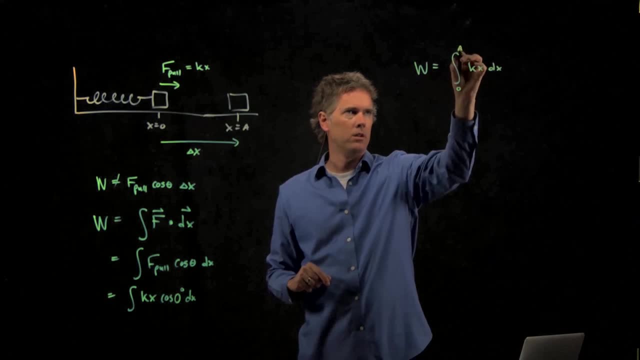 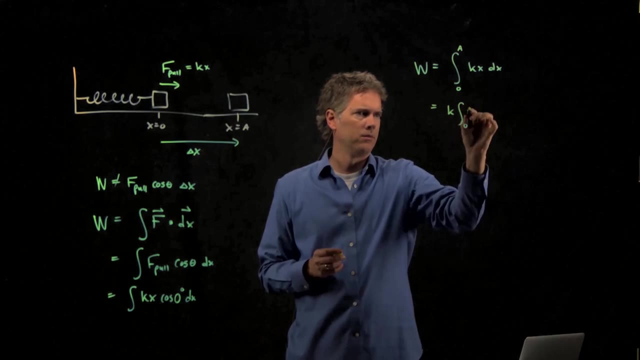 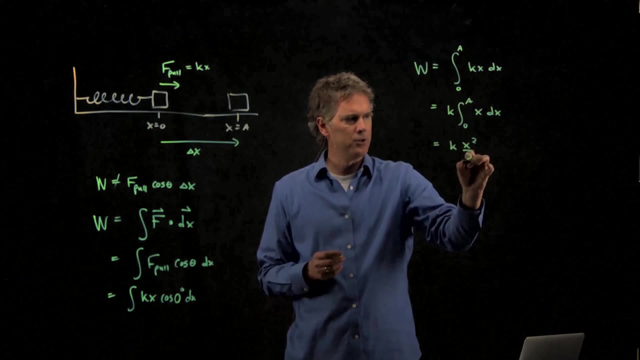 And we've gone from x equals zero to x equals a. k is a constant, So that comes out in front of the integral Integral. We know how to integrate x- dx. We just get x squared over two. We're going to evaluate that between zero and a. 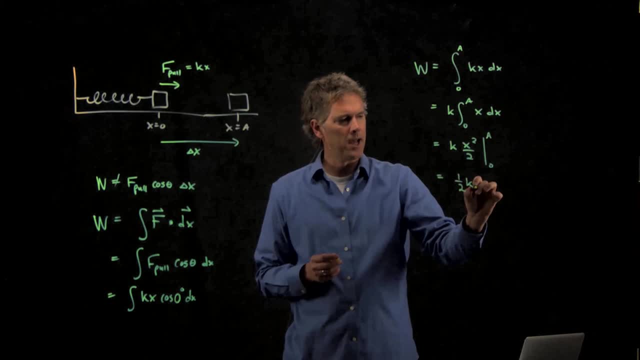 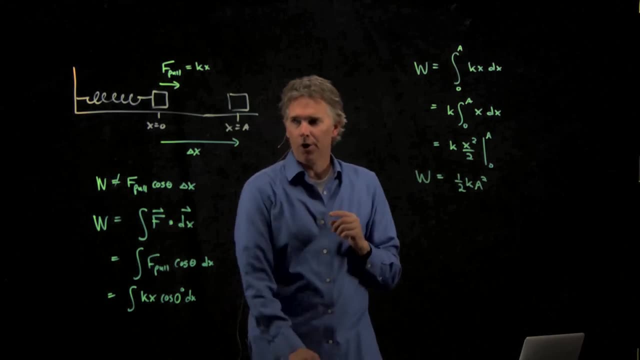 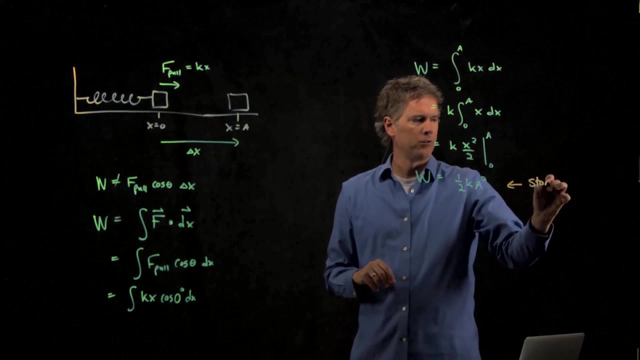 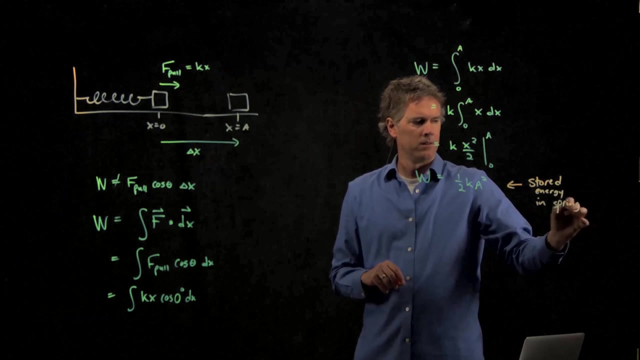 The zero is going to go away And we just get one half k a squared. That was the work that you did stretching out the spring And therefore it is also the stored energy In the spring, And you did work stretching it out, which means that energy had to go somewhere. 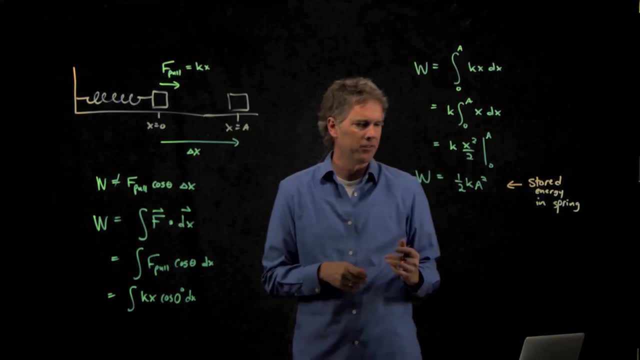 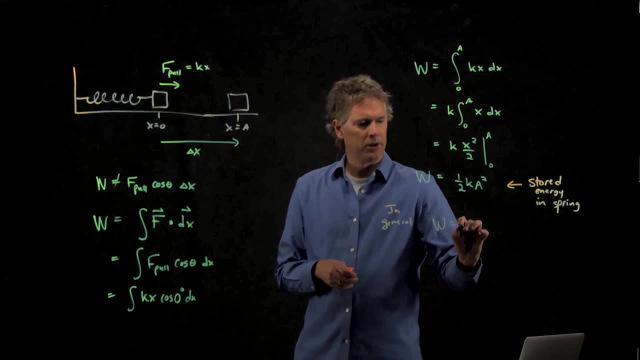 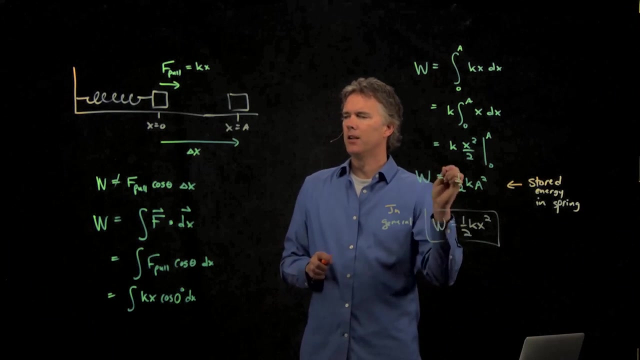 Where did it go? It went into the stretched spring itself, And we know what this is. in general, The work is one half kx squared And we saw that before. That's the energy in a spring. Where did it come from?